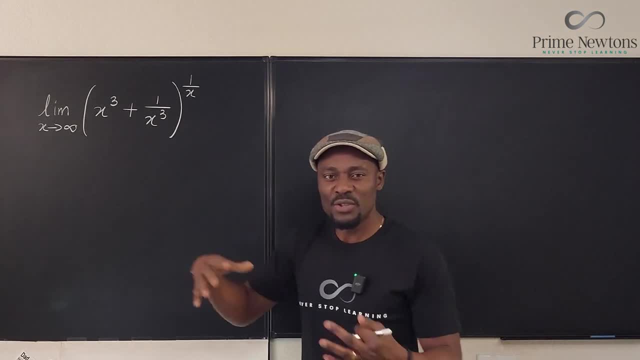 I start thinking I need to be able to write this in terms of the typical definition of Euler's number, which is E, because this is how we came about Euler's number originally. But this problem appears to not obey that rule. It's just going its own way. So what you do first whenever you get, 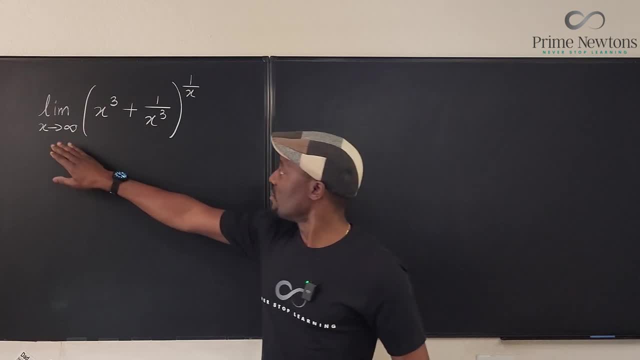 a problem where your limit is approaching infinity. well, what you want to do is see if it's possible for you to just have an idea of what's going on. Remember, you cannot plug in infinity So you can say, as x goes to infinity. 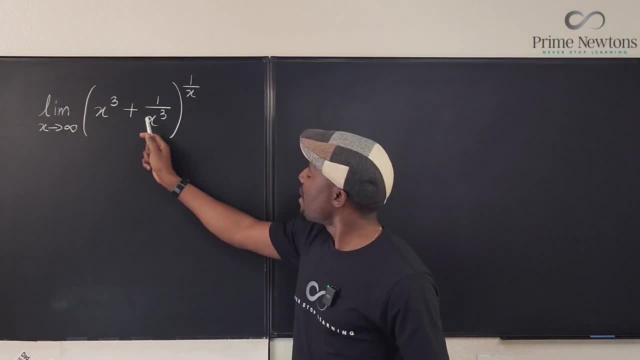 x cubed is going to go to infinity, but 1 over x cubed is going to go to 0. So you're going to have a situation of infinity plus 0, which is going to give you infinity. And then, when you 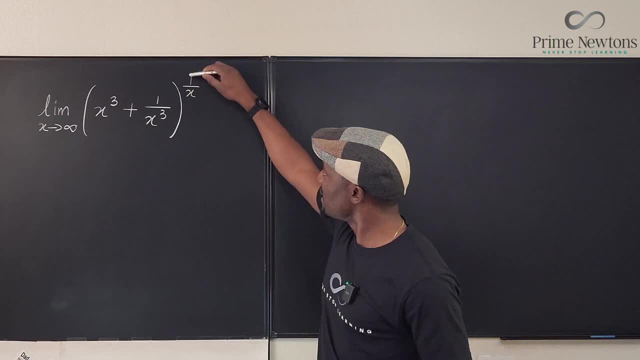 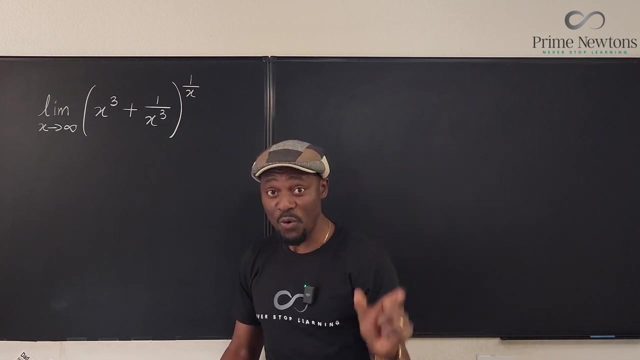 go to the exponent, it's going to be, as x goes to infinity, this goes to 0. So you have a situation of infinity raised to power 0. Well, infinity to 0 is what we call the indeterminate form. So you cannot say you have an answer because it's infinity to 0. So this means it's either you do. 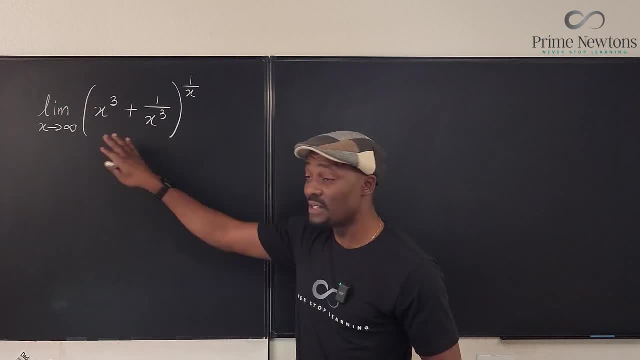 algebraic manipulations, or you have to rewrite this expression as a rational function, as a fraction, okay, And then apply L'Hopital's rule where necessary. So, looking at this, I think L'Hopital's rule is the way out. Let's get into it. 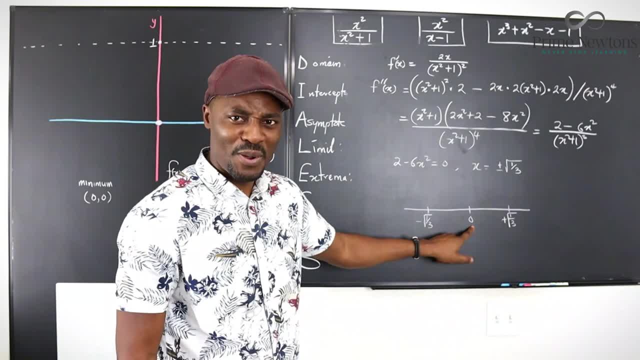 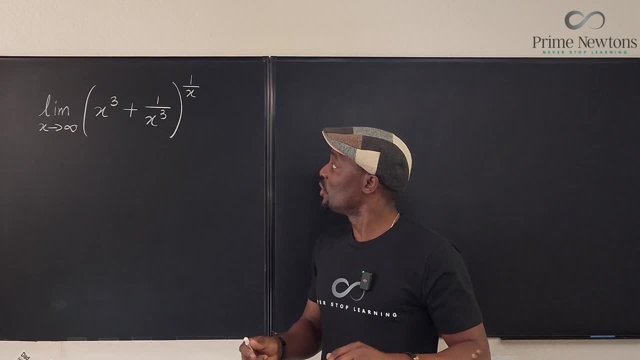 So in order to use L'Hopital's rule, it is necessary to write this as a fraction, But this doesn't look like a single fraction. This is an exponential expression. So I have to introduce natural law just to take this guy down. You always need to take this guy down, And what do I do? 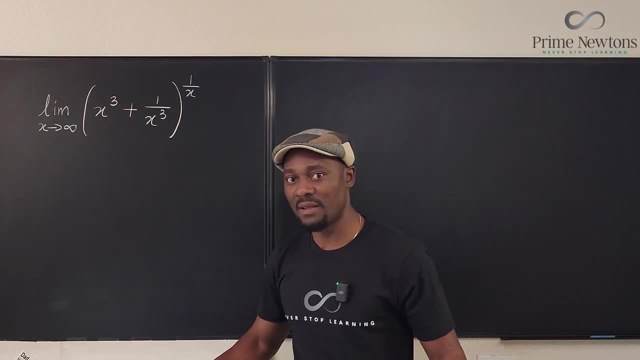 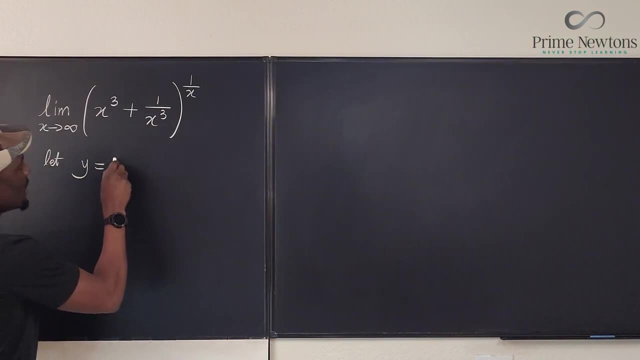 I need to say let this whole thing be equal to y. okay, So we're going to say let y be equal to this expression: x cubed plus 1 over x, cubed raised to power 1 over x. Before I go on, let me take the natural log of y. The natural log of y is going to be the natural 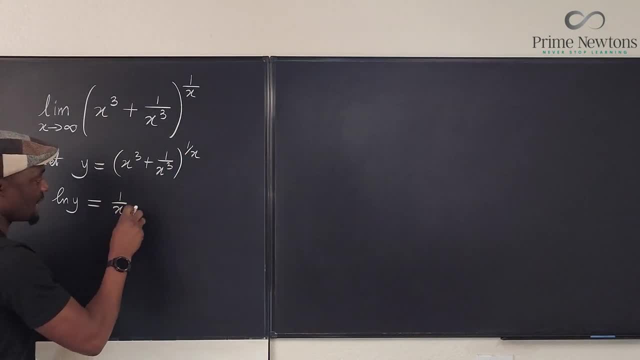 log of this, which means this comes down: It's going to be 1 over x times the natural log of x cubed. Nice, Okay, I'm not taking the limit yet. I don't want to take the limit yet because what I 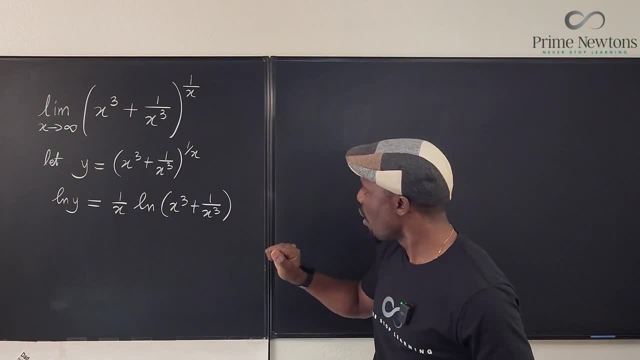 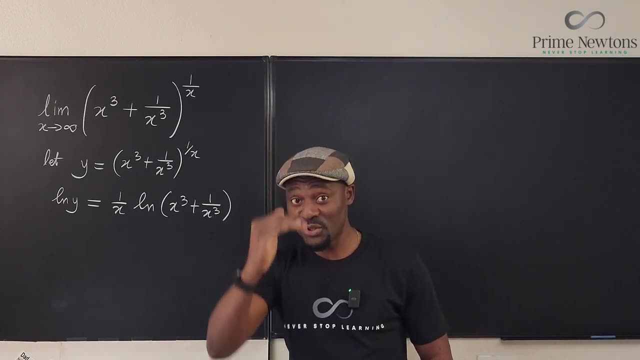 want to do is: I want to see what I have, what's going on. Remember, the mission is to use L'Hopital's rule, And for you to use L'Hopital's rule, you have to have a rational function, And that rational 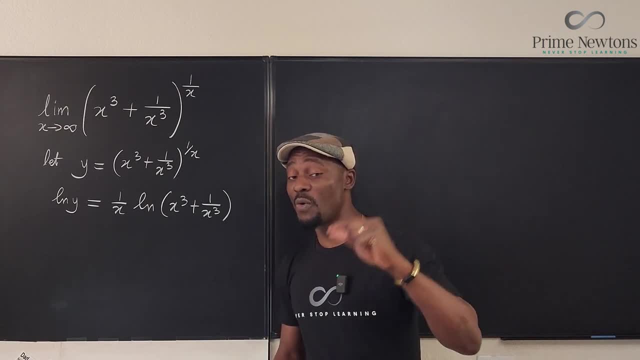 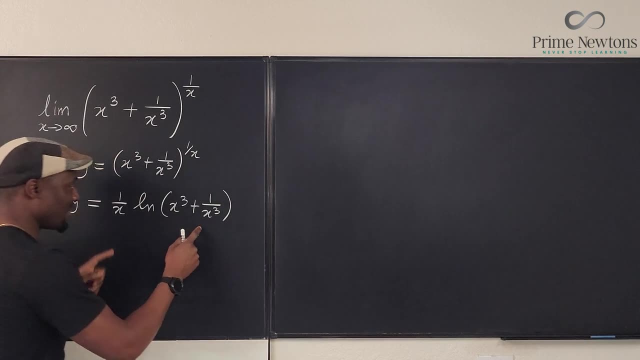 function is such that when you take the limit, you have to have 0 over 0 or infinity over infinity before you can use L'Hopital's rule. So here I found a little bit of a problem. I found a little bit of a problem. I found my secret, because I can write this expression on the right as the natural. 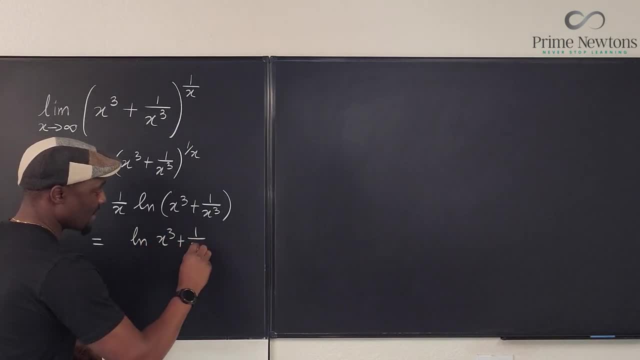 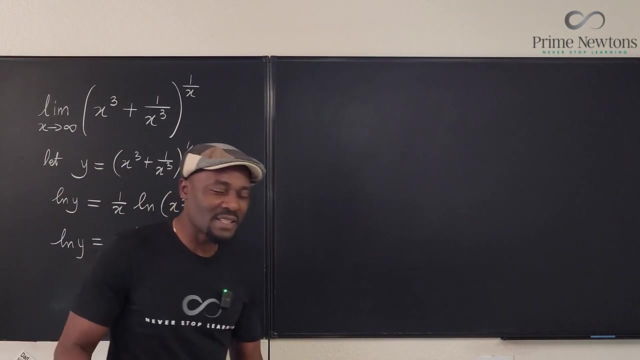 log of x cubed plus 1 over x cubed divided by x. You see, this x is now under all of them. So now I have a rational function and this is my natural log of y. So what I can do is now make an attempt. 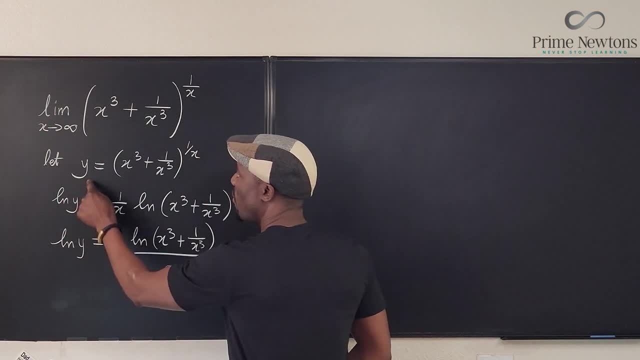 at taking the limit, just as the original problem was. Remember, y is all of this. So if I take the limit of y, I can take the limit of y. So I can take the limit of y and I can take the limit of. 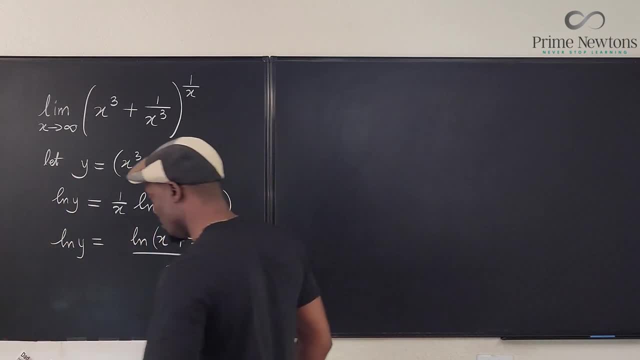 y. Or if I take the limit of the left-hand side, let's just take the limit of both sides, So I can say that the limit as x goes to infinity of the natural log of y, it will also be the limit I'm. 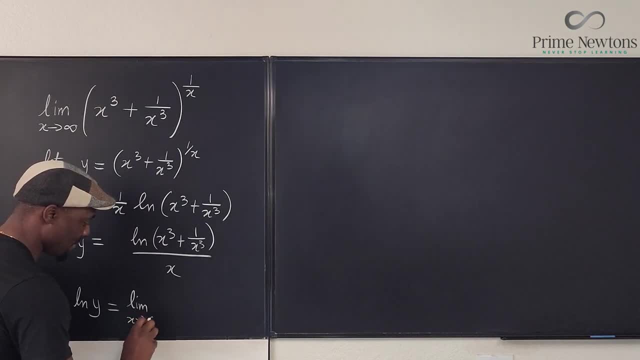 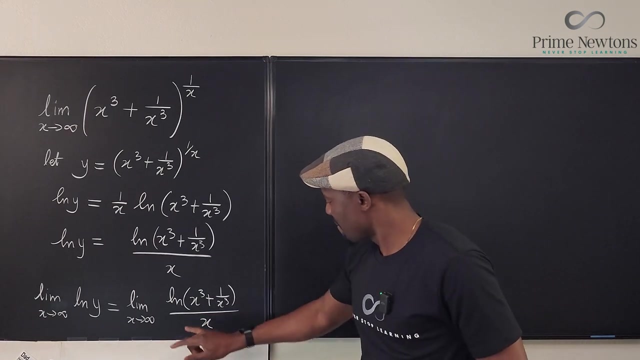 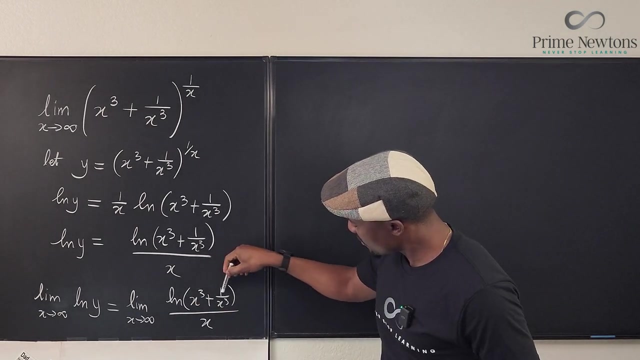 taking here the limit, as x goes to infinity, of the natural log of x cubed plus 1 over x cubed divided by x. So this is where I start thinking mathematically. Now I got to say: as x goes to infinity, what's going on here? This goes to infinity, this goes. 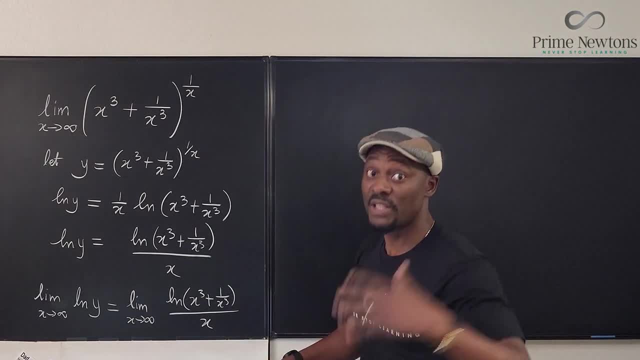 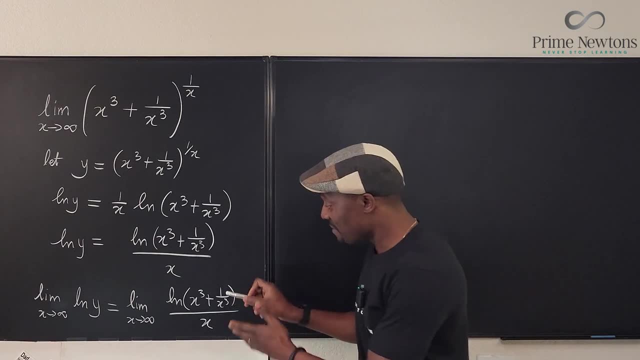 to zero. So I have the natural log of infinity, which goes to infinity right, And this also goes to infinity. So yay, I have found my infinity over infinity situation. So now I'm going to stop focusing on the left-hand side. My focus is on the right, If I can get a limit on the right. 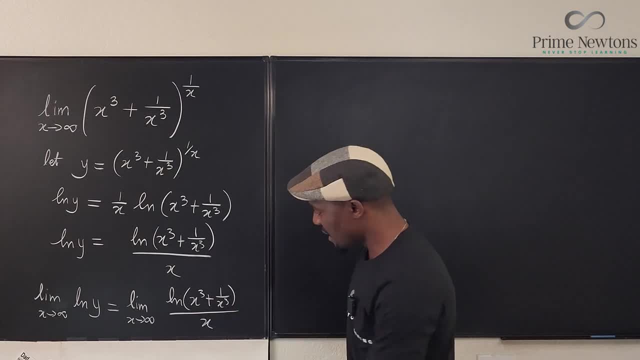 I can translate. I can translate it to the other side. So how do I take this limit? L'Hopital's rule. So by L'Hopital's rule I can say I will take the derivative of the top and then I take the derivative of the bottom. 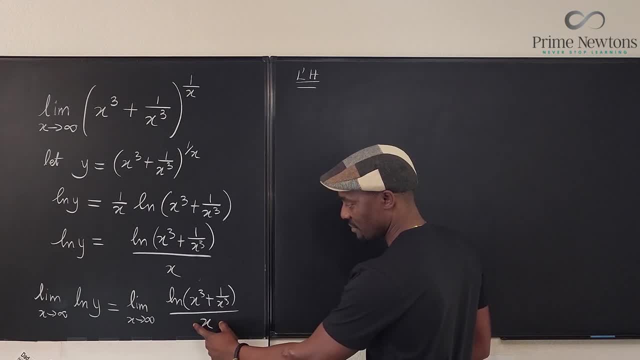 But obviously the derivative of this bottom is 1, right, So let's take the derivative of the top. So this is going to be equal to: if I differentiate any natural log function, what do I get? I'm going to get the derivative of the top. So I'm going to get the derivative of the bottom. So I'm going to. 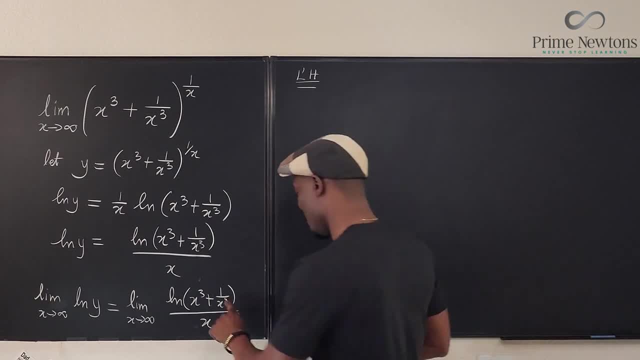 get the derivative of the argument divided by the argument. Let's do this quickly. So if I take the derivative of this, it's going to be- let's write it here- x cubed. This is going to be plus x to the. 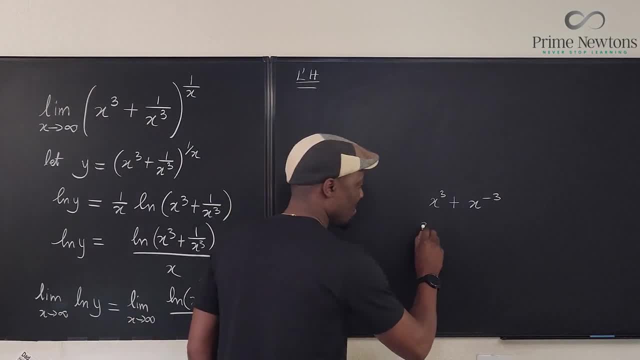 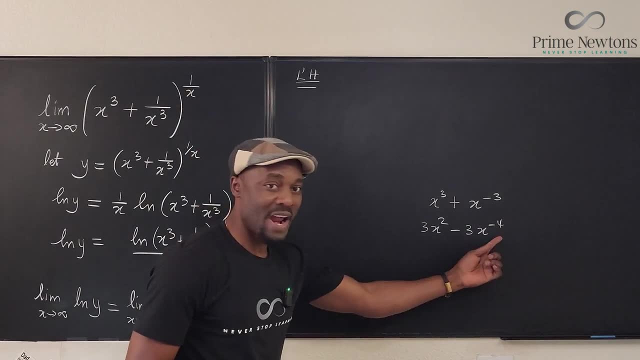 negative 3.. So we want to take the derivative of this. It's going to be 3x squared. This is minus 3x to the negative 4.. Okay, that's what you have, And if you write this out, it's going to look like: 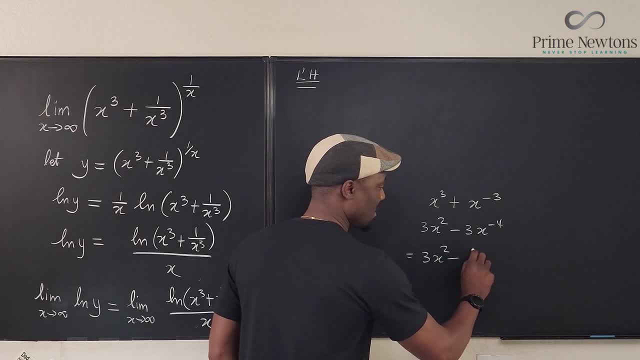 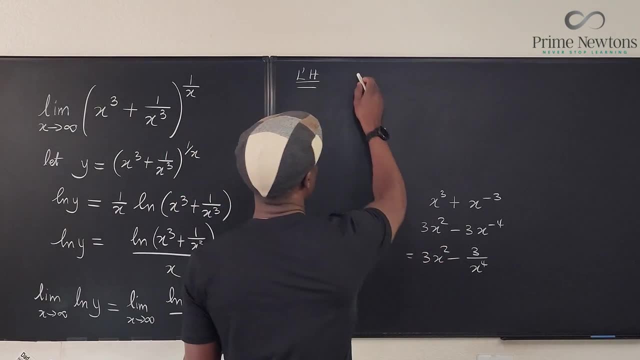 this: This is 3x squared, minus 3 over x to the fourth. This is minus 3x to the negative 4.. This is the derivative. So we're going to take the derivative of this. It's going to be 3x squared. 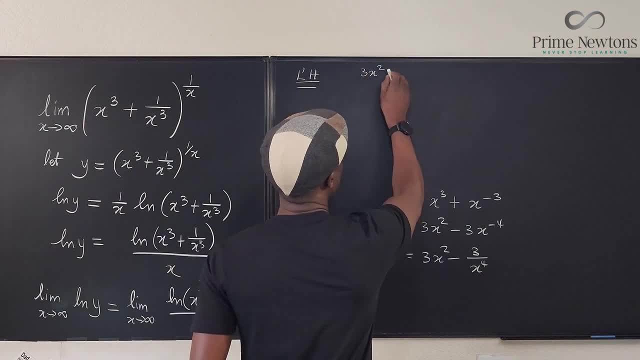 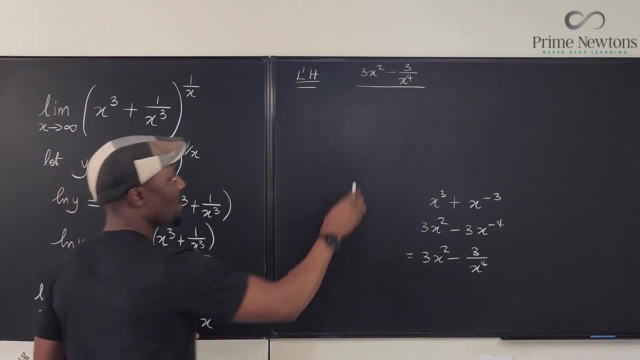 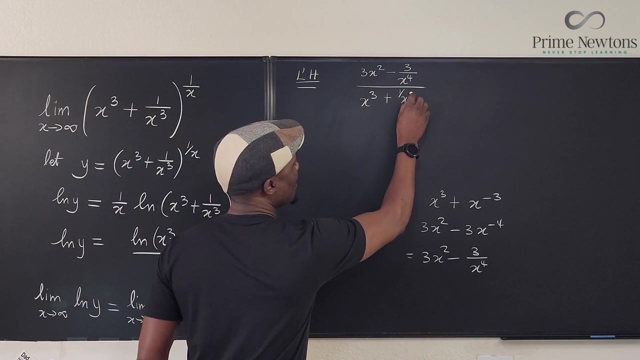 minus 3 over x to the fourth, divided by the argument itself, which is x cubed plus 1 over x, plus 1 over x to the third. Okay, let's write it that way: 1 over x to the third. 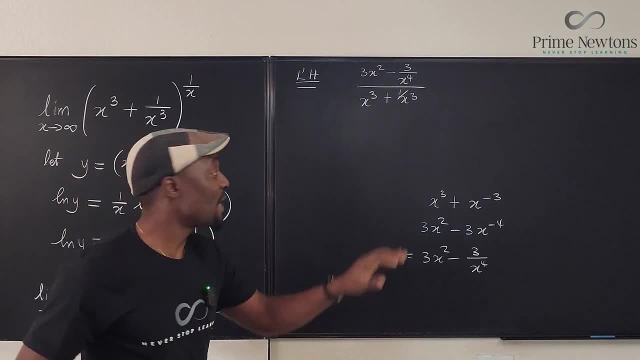 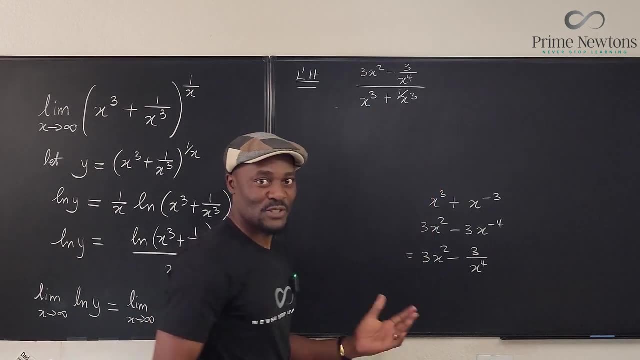 Now, that's the derivative of the argument. So we're going to take the derivative of this. It's going to be the derivative of the top. only, I just took the derivative of the top. What's the derivative of the bottom? It's 1.. So I'm going to divide this by 1, but there's no point writing that, And this is: 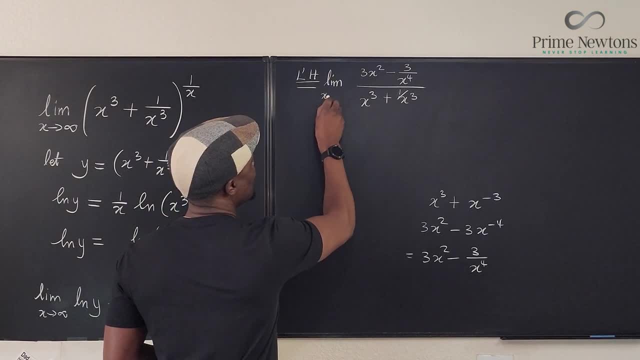 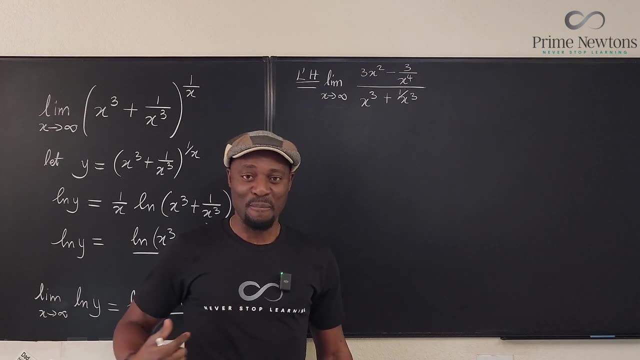 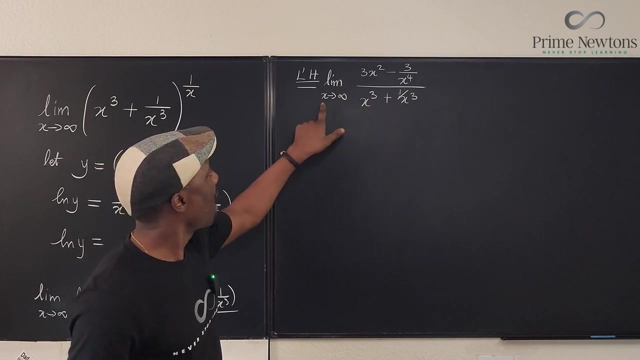 what we have, the limit as x goes to infinity. By the way, leave a comment in the comment section if you like my new shirt. Now we need to try and see whether we can evaluate the limit If we try to see what's going on as x goes to infinity. 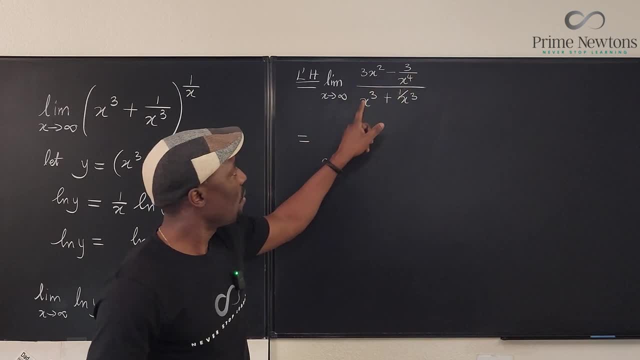 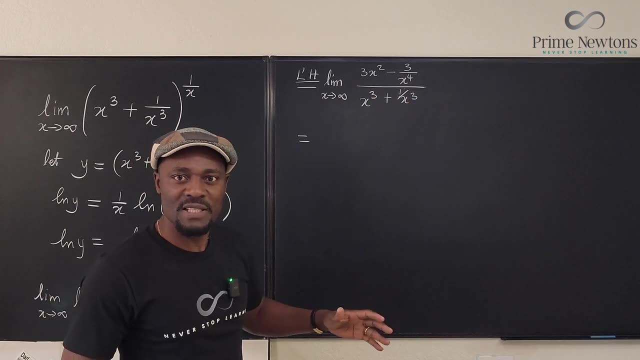 this goes to infinity. So we're going to try and see whether we can evaluate the limit If we try to see what's going on. as x goes to infinity, this goes to infinity. So this is infinity minus 0 over infinity plus. Ah, we can't do that. okay, It's still infinity over infinity, but we can do. 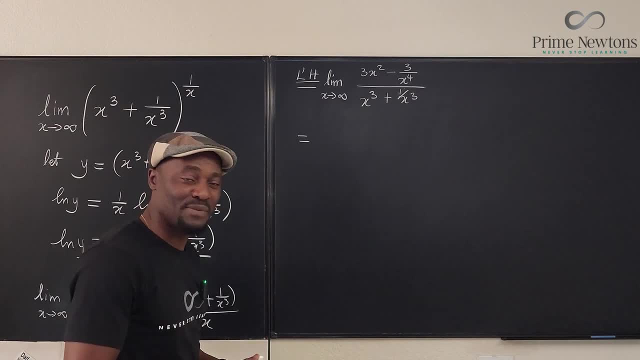 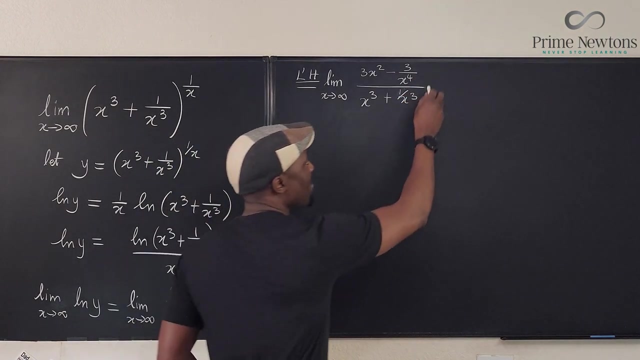 some simplification. right, Let's try and do some simplification, Because there's a fraction within a fraction. why don't we try to get rid of the fractions, okay? So if I want to get rid of these fractions, this denominator, I can multiply the top and bottom by x to the fourth. So what I'm 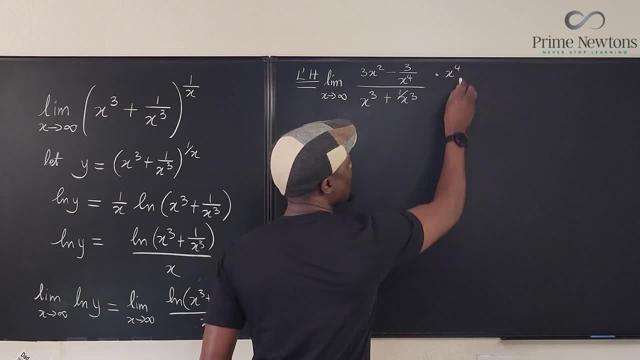 going to do is I'm going to multiply the top and bottom by x to the fourth. So what I'm going to do is I'm going to multiply this by x to the fourth and I'm going to multiply this also by x to the. 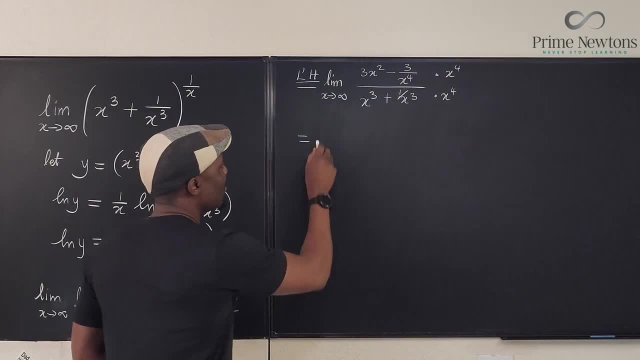 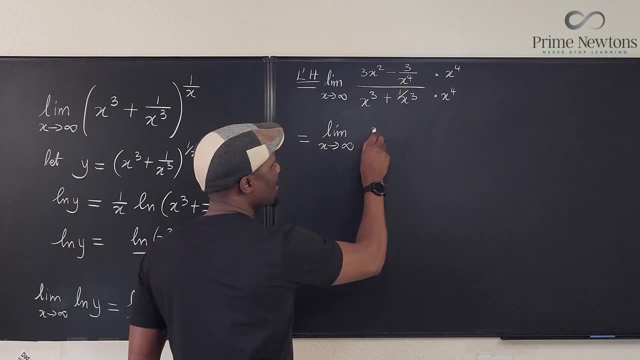 fourth. So I'm not changing anything. See what happens. This becomes the limit as x goes to infinity of. This is going to multiply this. You're going to get 3x. to the sixth: This is going to multiply this. You get minus, just 3.. Oh nice, That's cool. 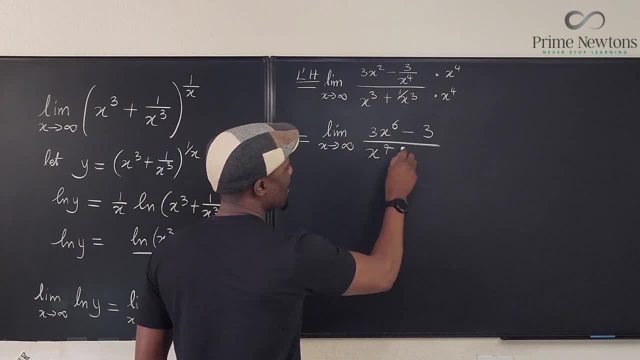 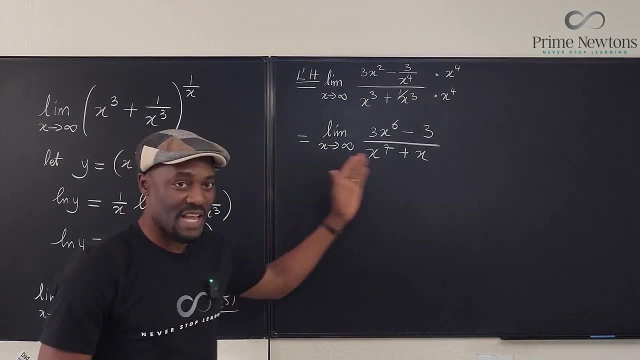 Multiply this by x to the fourth: You're going to get x to the seventh. Multiply this by x to the fourth: You're going to get x plus x. Nice, Now can we take this limit? Looks like we can, because now we have just a simple rational expression: How do you take the limit of? 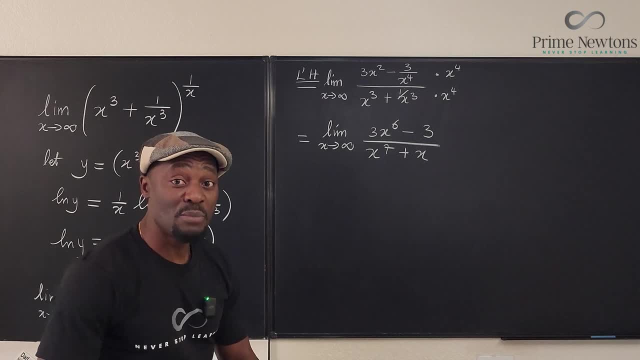 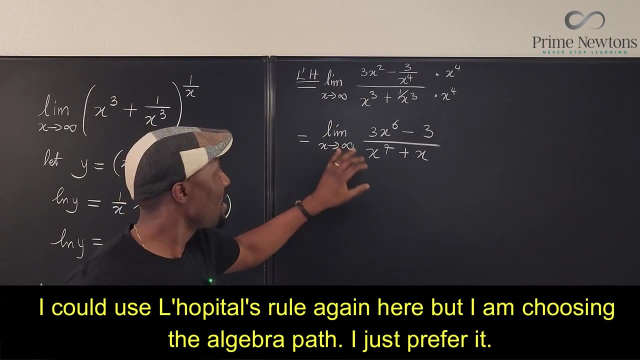 rational expressions as x goes to infinity. Well, remember, the strategy is to look at the denominator and see which one has the highest degree. The highest degree in the denominator is: remember it's the denominator, not all of it. We get x to the seventh. 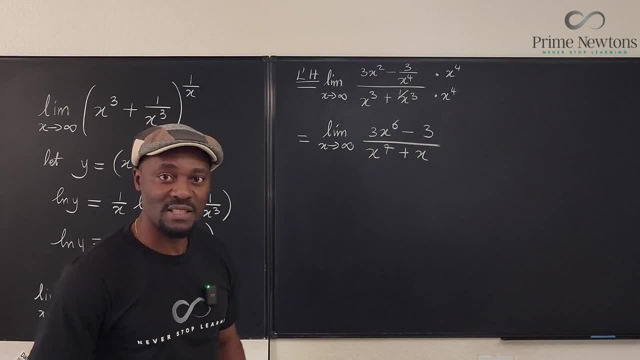 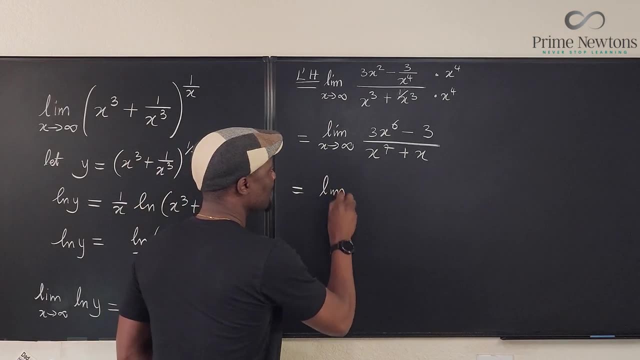 Use x to the seventh to divide every term. you see, in this limit, Every time you have infinity. That's the strategy. So what do we have? This is going to be equal to the limit, as x goes to infinity of What do we have here? We're going to have Oh, 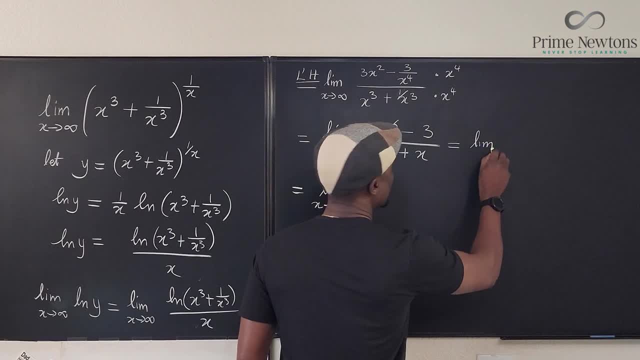 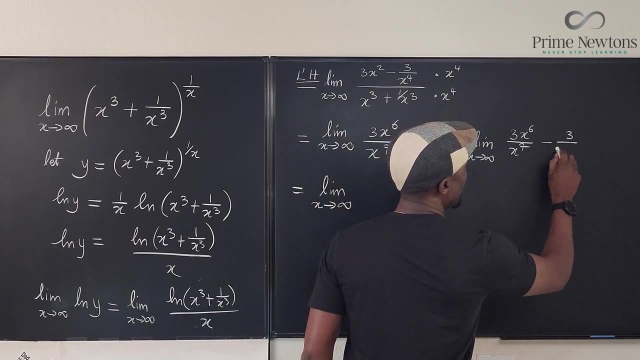 maybe I should write it here. Let's go this way. This is going to be the limit, as x goes to infinity. If I divide everything by x to the seventh, this is going to become 6 over x to the seventh, minus 3 over x to the seventh. An alternative strategy is to just: 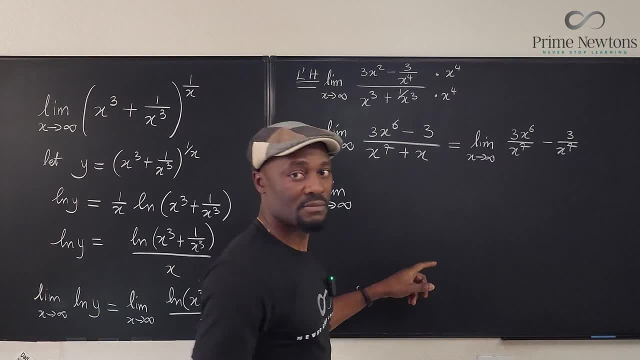 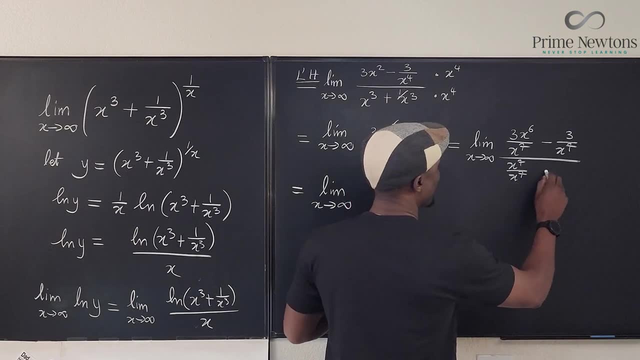 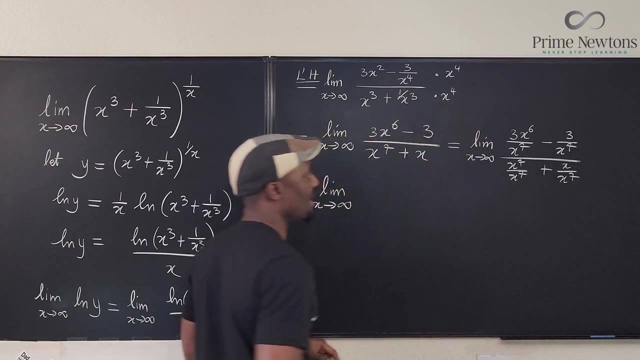 factor out whatever is common to the top and bottom. Some people like doing that, I like doing this. Divided by x to the seventh over x to the seventh, plus What do I have here? I have x over x to the seventh. Okay, What will this become? Well, look at this. This is going to become 3 over. 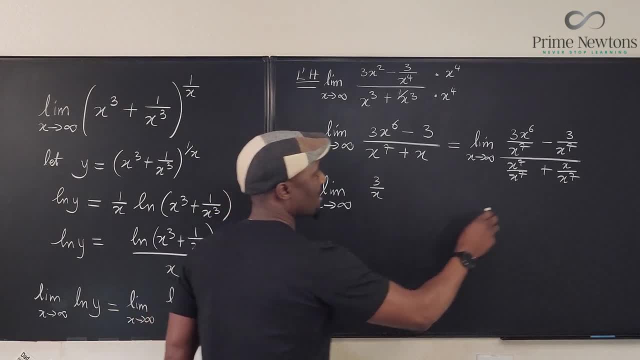 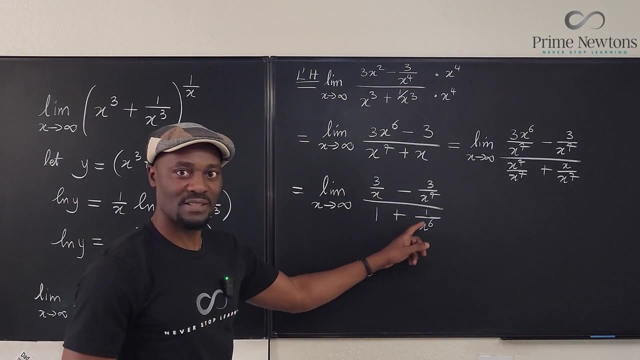 x. This is 3 divided by x. This is going to be minus 3 over x to the seventh. What do I have here? I got 1.. What do I have here? I got 1 over x to the sixth. Nice. So if we take this limit now, 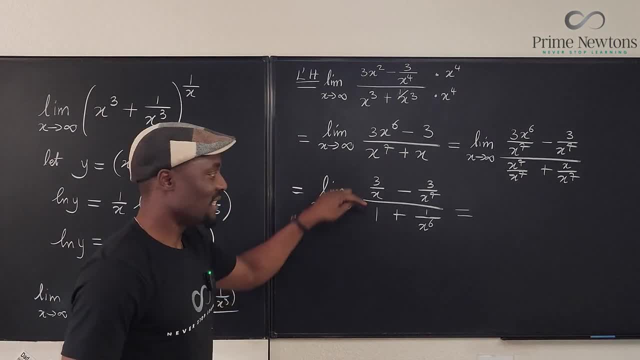 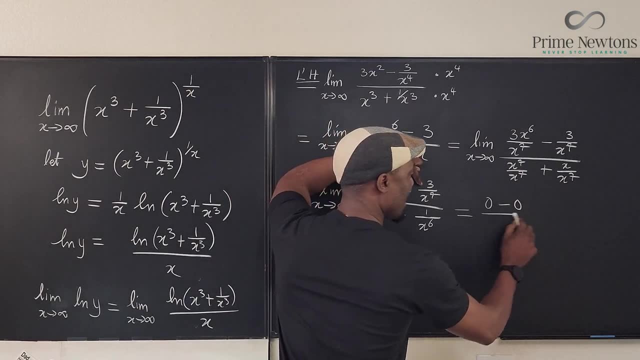 nice. As x goes to infinity, this goes to zero. As x goes to infinity, this goes to zero. This is 1, and this goes to zero. So we have 0 over 1,, which is equal to zero. So this limit on. 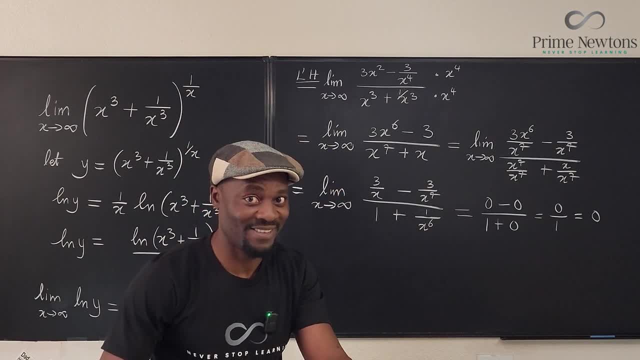 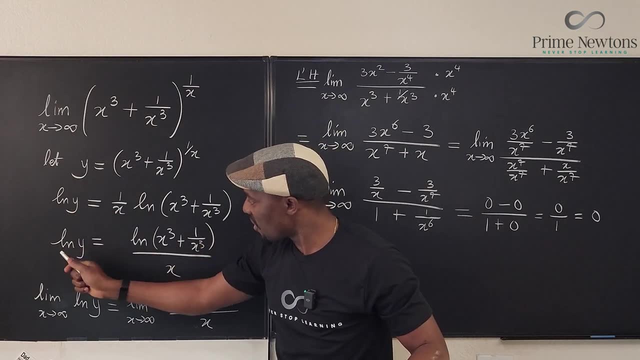 the right-hand side is zero. It is not your answer. Remember that the limit we took on the left is not the limit of y. We took the limit of the natural log of y. So this is what you're going to say. You're going to say so. 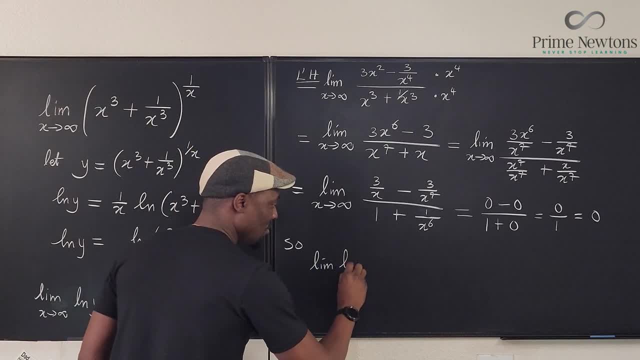 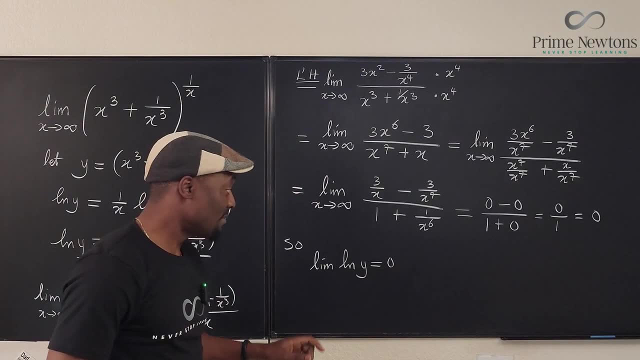 The limit of the natural log of y is equal to zero. What does that mean? Well, that simply means you can move this limit. Oh, as x goes to infinity. I'm sorry, This implies Okay. So one of the laws of limits is: the limit of a function is the function of the limit. 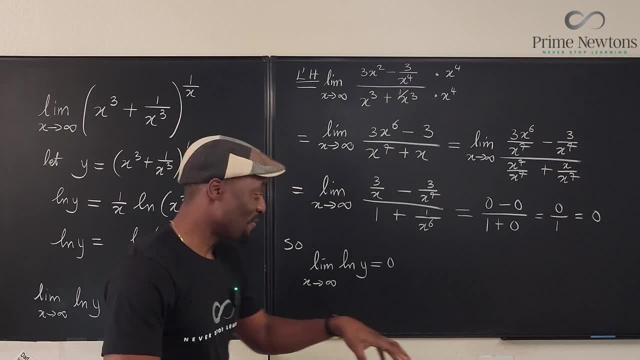 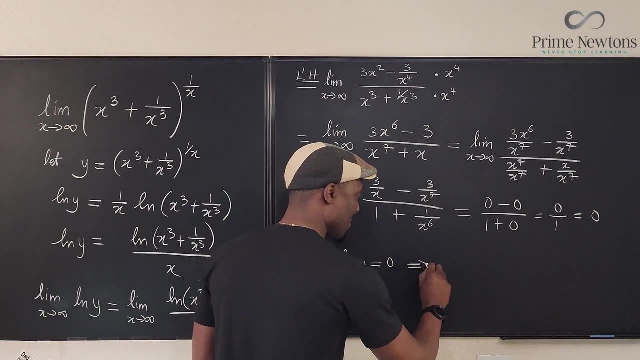 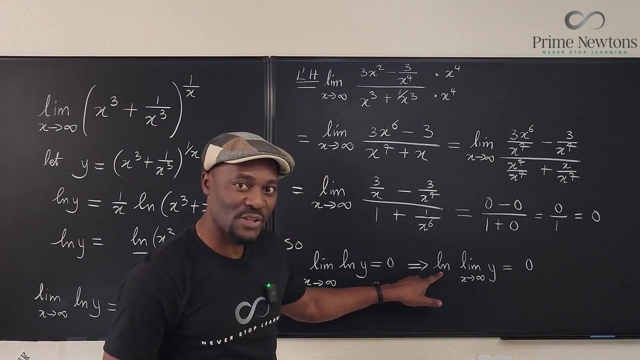 as long as the limit exists. Okay, So what we're going to do is we're going to move this limit right in there. So this is the same thing as the natural log of the limit. as x goes to infinity of y is equal to zero. And what does this mean? How do we get rid of this natural log? We raise: 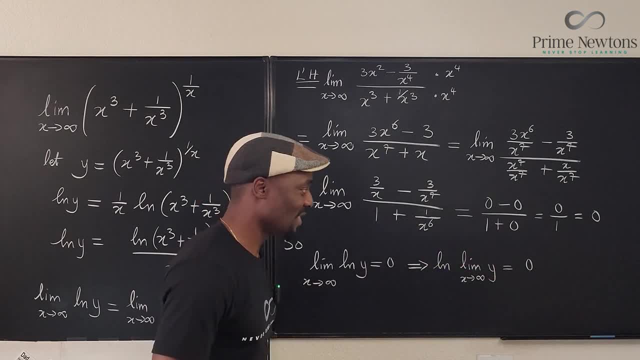 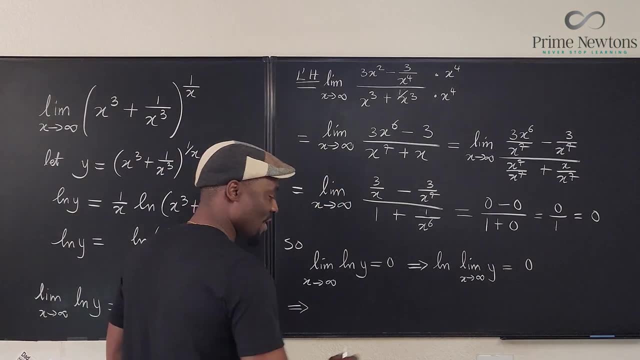 both. We e both sides. That's what I like to say. So if you take the e of both sides, this implies that If you get rid of natural log by taking the e of both sides- I'm going to do it here, You do it here and you do it here. 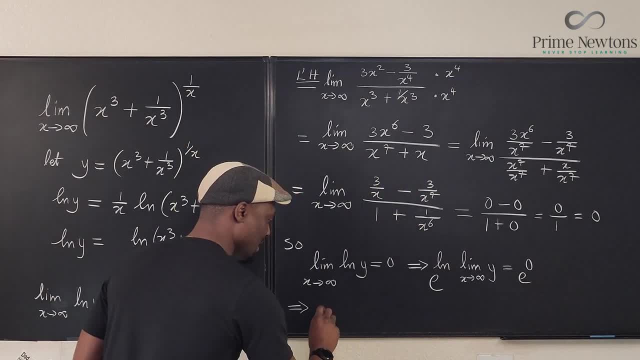 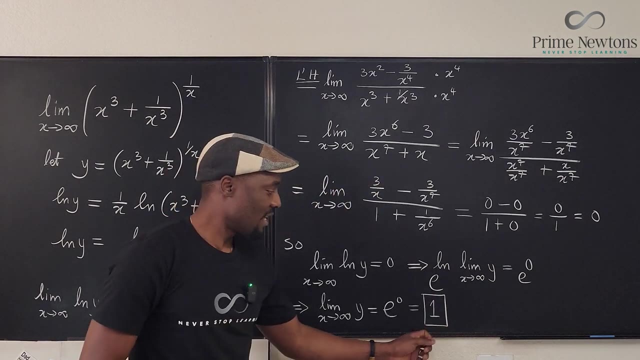 You see what happens. What is left on the left-hand side is the limit, as x goes to infinity, of y is equal to e to the zero. What is e to the zero Equals one. So this limit, ultimately, is one. Never stop learning.